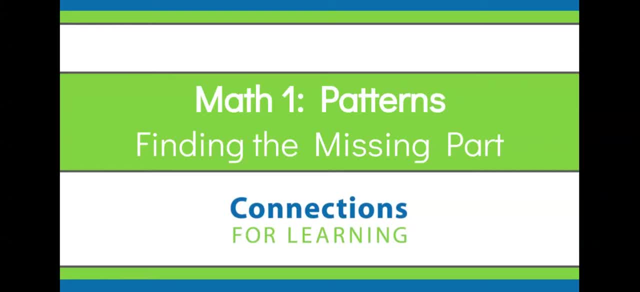 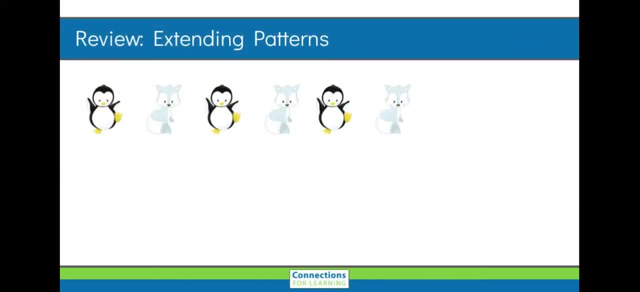 Please add punctuation in the appropriate places. And if I look at the pattern, there, after every fox comes a penguin. So if you guessed penguin you would be correct. And then what comes after the penguin? Well, after every penguin in this pattern, we see another fox. 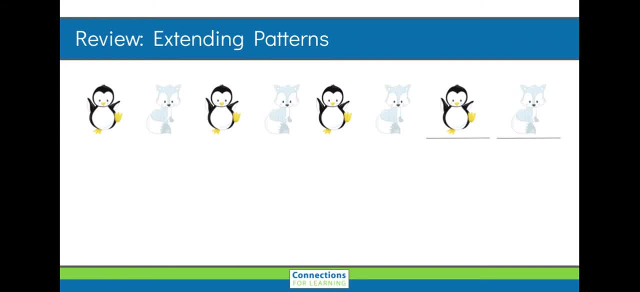 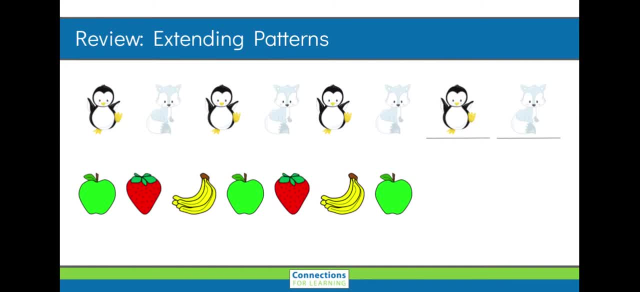 Let's take a look at another example. Here we have an apple, a strawberry and a banana. An apple, a strawberry and a banana, An apple and a. Well, if you guessed strawberry, you got it. And after every strawberry in our pattern, we see a banana. 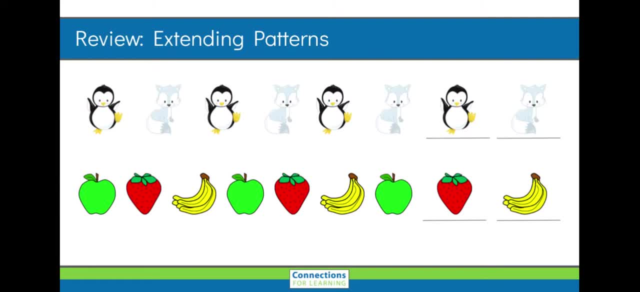 Now we can go back again to the beginning of our pattern and see if our answer follows the pattern. that's here We have an apple, a strawberry and a banana, And then our pattern starts over with an apple, a strawberry and a banana. 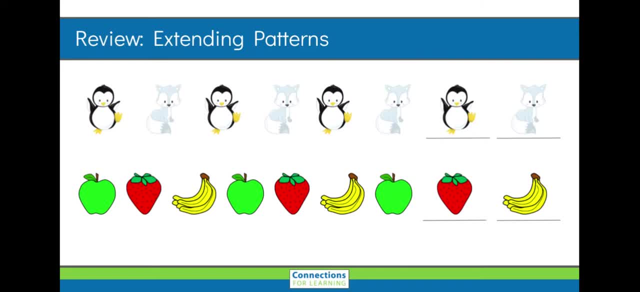 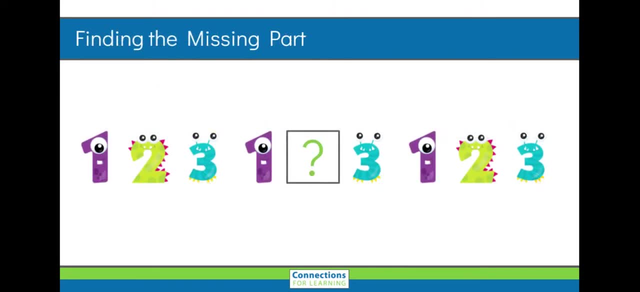 And then an apple, a strawberry and a banana. That looks great. Now, when we're looking at finding the missing part, we're looking for what's missing in the middle of our pattern. So instead of making our pattern longer, we're going to try to complete it. 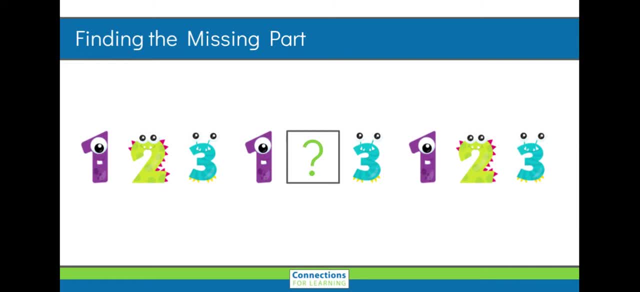 Now, if I read this pattern, which is always a great place to start, I'm going to see that we have a 1, and then a 2, and then a 3, and then another 1.. Oh, something we're not sure. 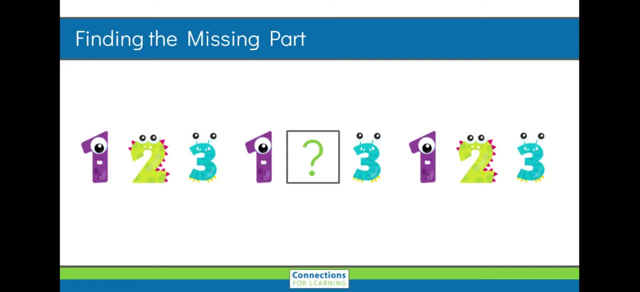 A 3, then a 1, then a 2, then a 3.. Well, I think you can all count to 3.. So if you guessed the 2 is missing, you would be right. We have a 1.. 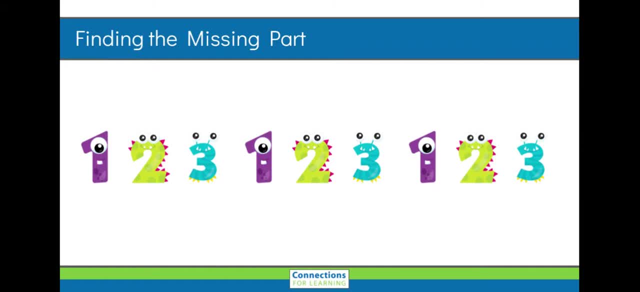 We have a 1, 2, 3,, a 1, 2, 3, and a 1, 2, 3.. That's a great job. Now, what do we do if we have two missing parts? 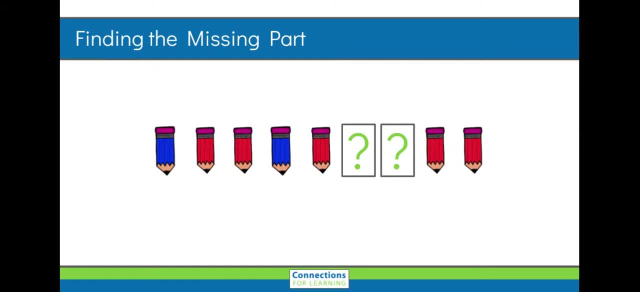 Well, again, we can start at the beginning of our pattern and we can read it out loud. We can use what we see in the pattern or we can read it as an A- B pattern, And we can try both of those here. 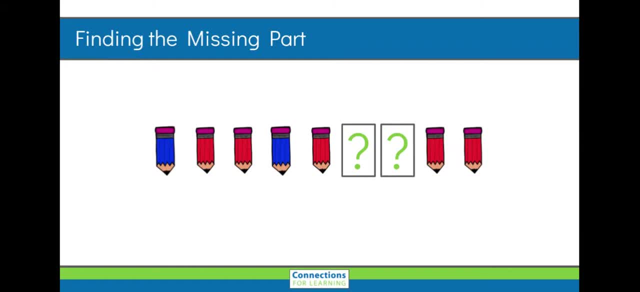 A blue and a red and a red, A blue and a red and a mm and a mm and a red and a red. Well, let's try A and B. We'll say blue as an A, red as a B. 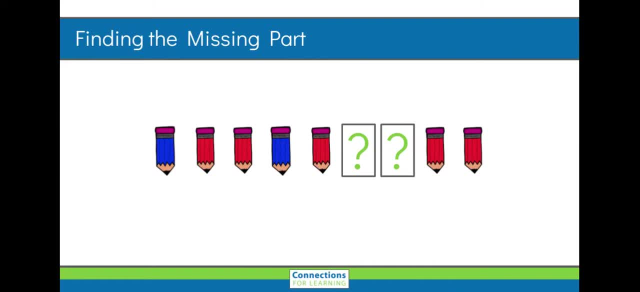 Let me see A, B, B. A B, mm, mm, B B. Well, when we extended patterns, we looked at what came just before, Just after the last one. So if I look here, I see a red pencil right before our unknown, and before that is a blue. 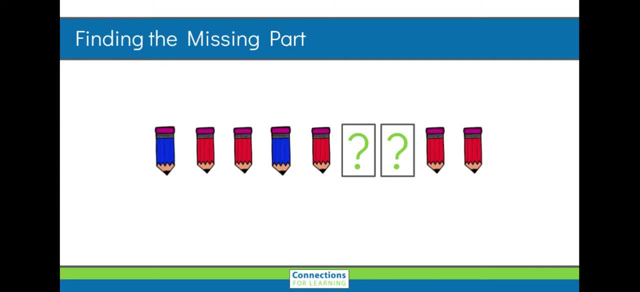 So I wonder if this is a blue and a red, just like the two that come before it. Well, let's read this pattern out loud: Blue, red, red, blue, red, blue. oh, blue, red, red, red. 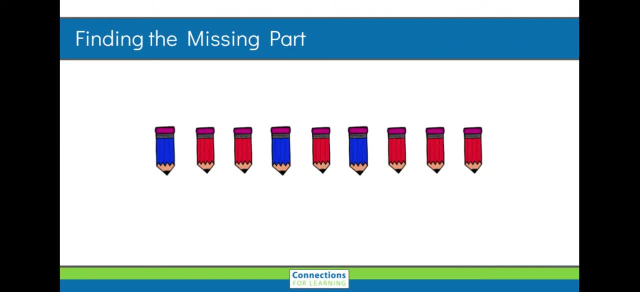 Uh-oh. So something doesn't look quite right here. I'm going to try again using letters and see if I can figure out what's going on. If I say blue is an A and red is a B, again we would read A, B, B. 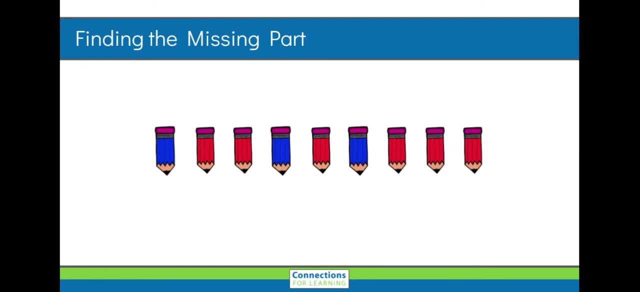 A, B, B. So the blue one should be a red one and the red one should be a blue one. Let's double check just to make sure. Blue red, red, blue red red, blue- red- red. 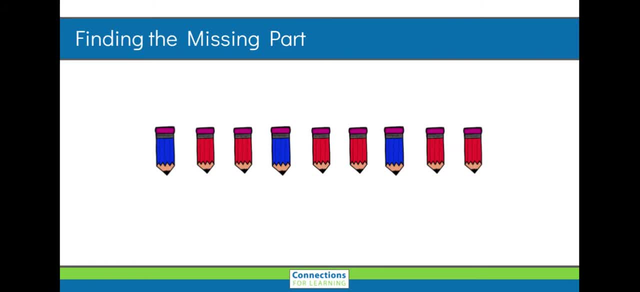 Oh, that sounds much better. Or we could read: A, B, B A, B, B, A, B B, Great job. Here's our last example for today, and this one might be a little bit trickier.